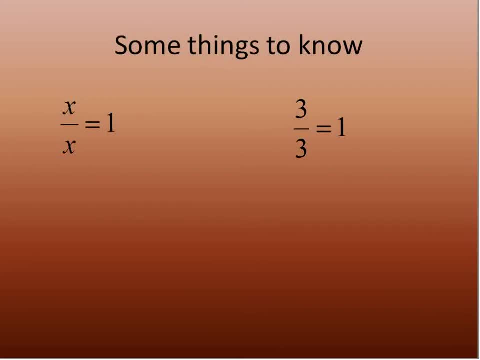 that. So you'll need to know this- that if you want to get rid of something or cancel something out, you divide by that same number. So three divided by three is one. Anything divided by itself is one. Also, you can rewrite a fraction of some number. 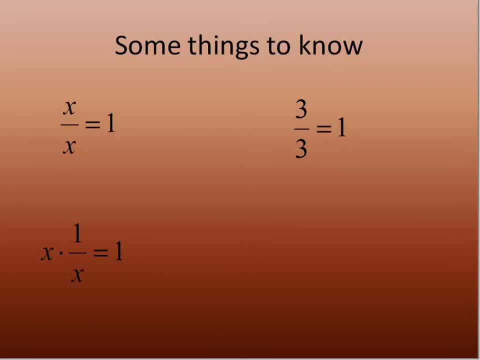 over and over again. So you can rewrite a fraction of some number over and over again. So you can rewrite a fraction of some number over and over itself, like x divided by x. You can rewrite that as x times one over x. Again, something that we are definitely going. 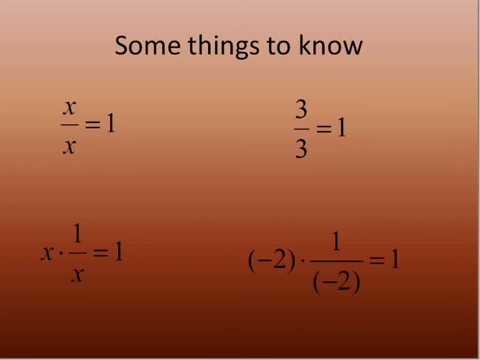 to use in the future and it relates somewhat to the idea of reciprocals, but definitely something you're going to need to know. So here's an example: If you have one over negative two, you multiply times negative two and then that would reduce down to being one. 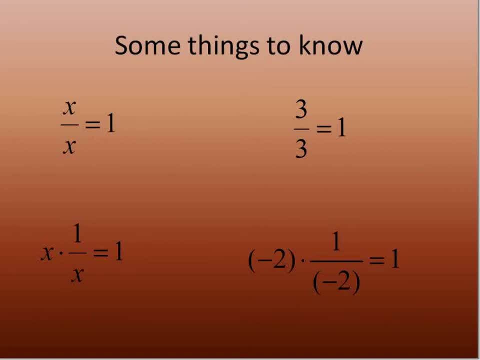 So we will see this later on and it relates to reciprocals a little bit. So let's talk first off what is a reciprocal. A reciprocal, also called a refliperical, is when you flip over a fraction. So two-thirds would be flipped over to become three over two. So the reciprocal 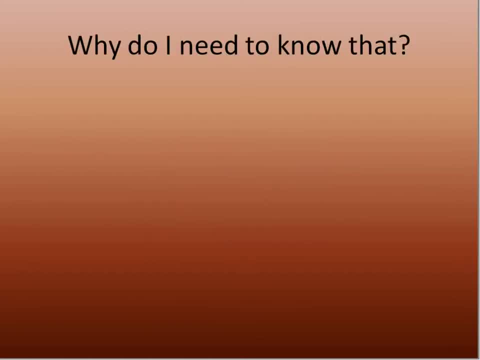 of two-thirds is three over two. Now we actually need to know that. It's really important that we know that, Because a fraction multiplied by its reciprocal is equal to one. Isn't that nice to know. So four over five times five over four is equal to one, And that's why you need to know. 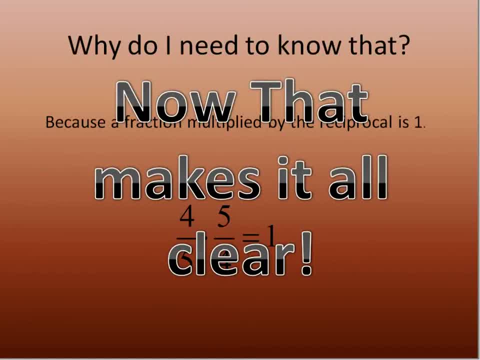 It's very important in your life. Huh What? All right, So, although what I said is true, that doesn't really answer your question of why you'll need to know it. So we will need to know it because you'll be multiplying by reciprocals and you'll be multiplying. 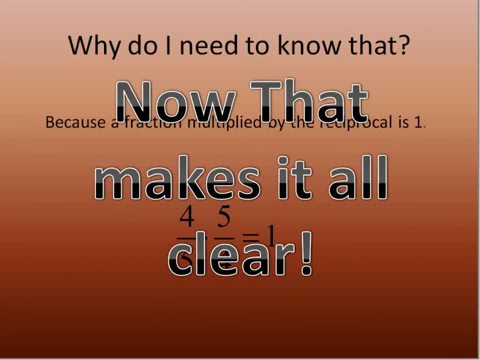 by fractions and you'll be removing fractions from equations. That's why you'll need to know about reciprocals, And also multiplying reciprocals does equal one, so that helps us to eliminate fractions when we're working with fractions equations. All right, So let's. 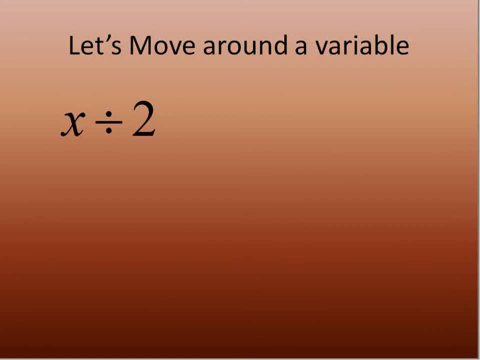 look again. we need to be very comfortable in algebra one. You need to be comfortable with the variable and moving it around. So to say, two or x divided by two is the same thing as X times one half right or x divided by two. Now, these two here are the rules that I said. 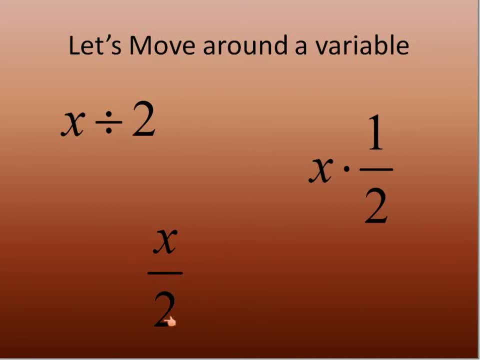 at the beginning. right, Something over something is the same thing as the numerator multiplied times that fraction: one over two. Also, this one is the same as what we do when we divide, and we're going to do this in a little bit. 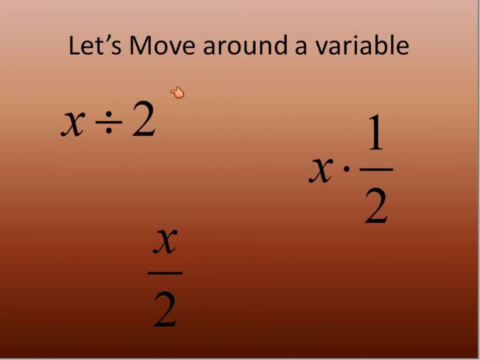 If you have something divided by something else, that's the same as saying the first number times the reciprocal, And two is like writing two over one. so the reciprocal is one over two And we'll look at some questions involving multiplying. You can change division. 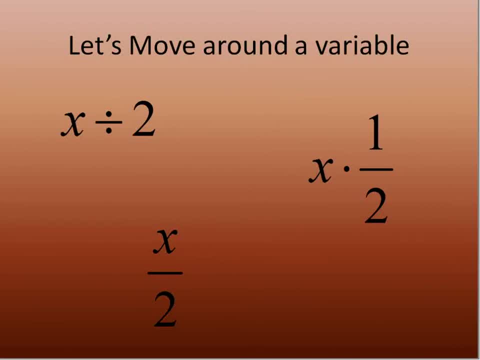 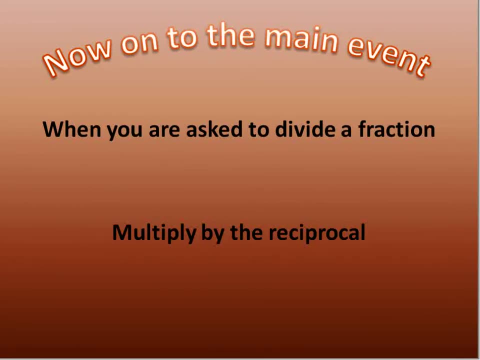 questions to being multiplying by the reciprocal. You often do that when you're dealing with fractions, So let's take a look at them- actually the main event, how to actually use these in some math situations- and see what we're doing. So when you're asked to divide a fraction, you would 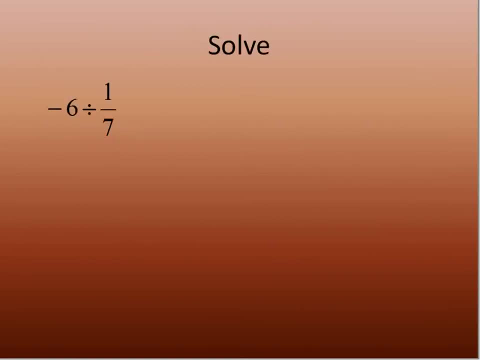 multiply by the reciprocal. it's exactly the same thing. So here's an example where we have negative 6 divided by 1 over 7.. What we're going to do is write negative 6 as a fraction- negative 6 over 1, and then it's divided by 1 over 7.. 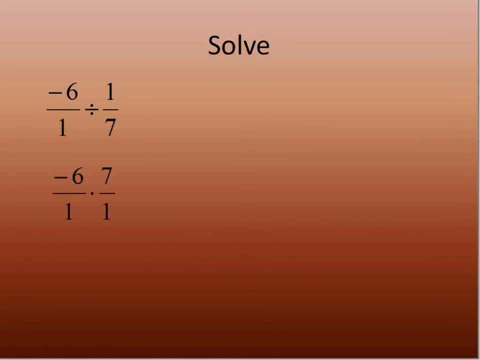 What we want to do is multiply by the reciprocal, so we flip over or we get the reciprocal of the second fraction and change it to multiplication. So now it's negative 6 over 1 times 7 over 1, and we can rewrite that you know something? 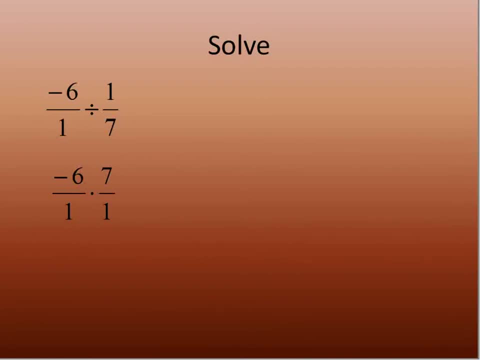 divided by 1 is just that number. so negative 6 divided by 1 is negative 6,. 7 divided by 1 is 7.. So that's the same as saying negative 6 times 7, which will give you a negative 42. So that's what you can do when you've got, when you start.